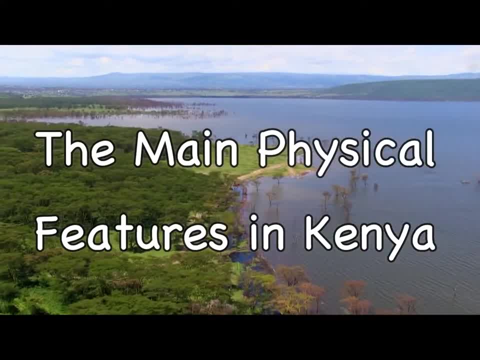 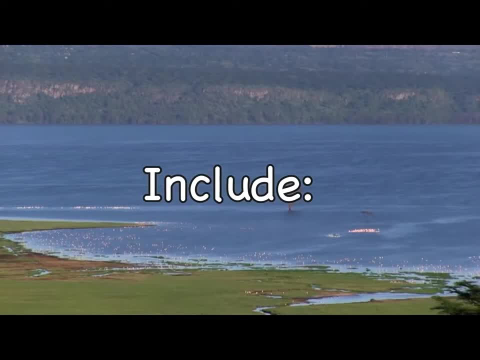 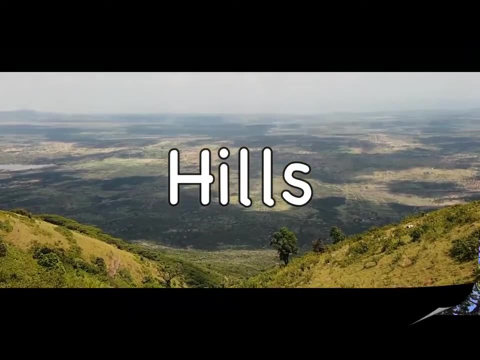 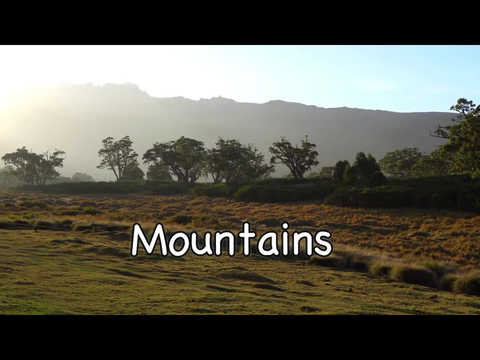 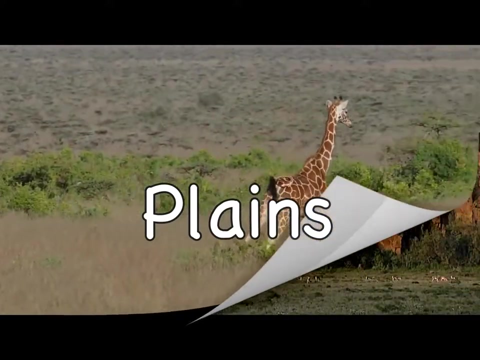 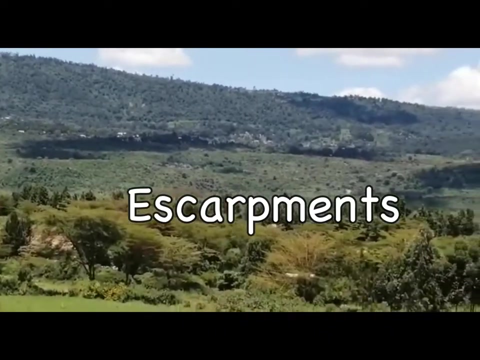 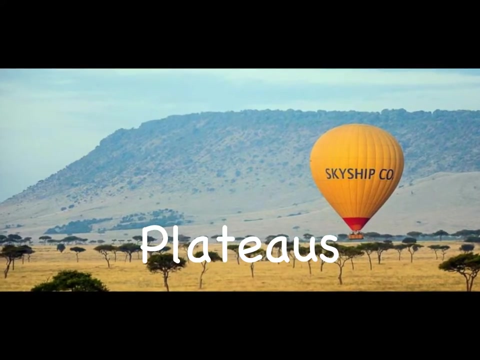 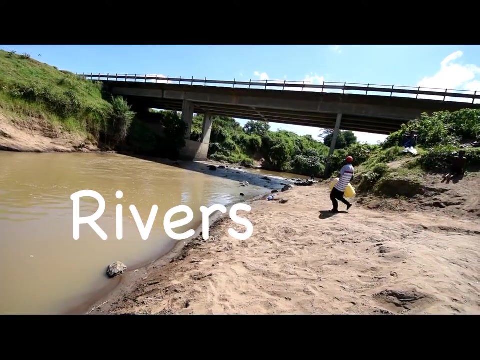 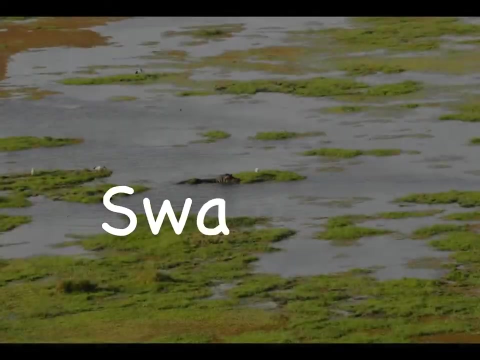 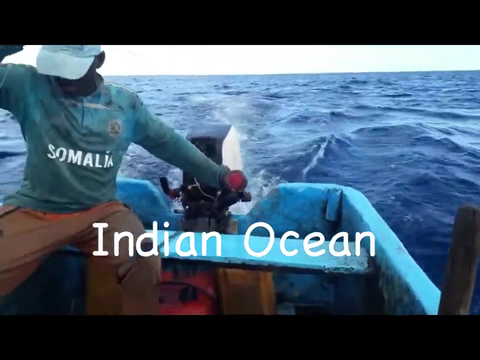 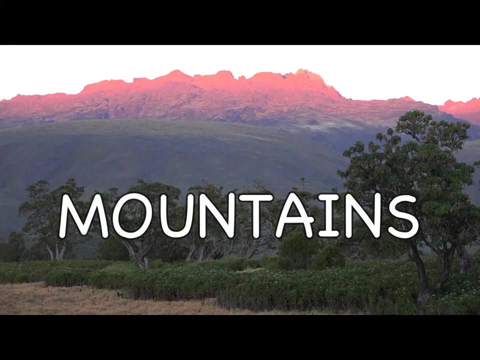 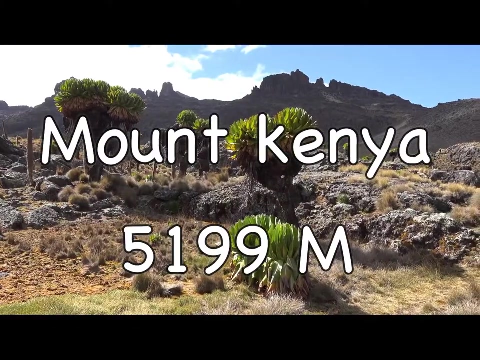 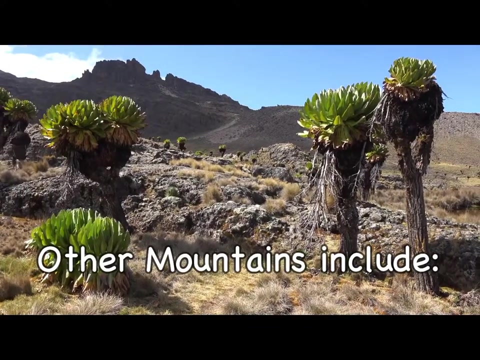 The main physical features in Kenya. The main physical features in Kenya include hills, mountains, plains, valleys, escapements, plateaus, rivers, lakes, swamps, rivers and an ocean. mountains- The highest mountain is Mount Kenya, which is 5,199 meters. Other mountains include Mount Elgon. 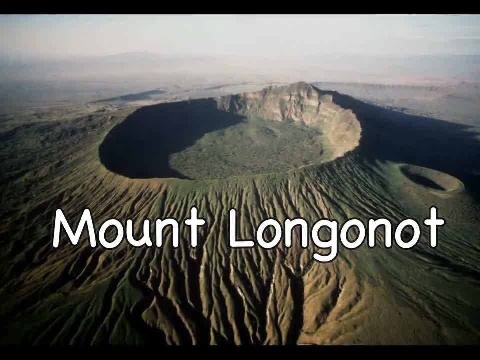 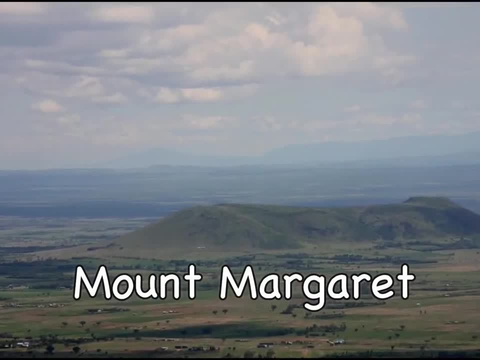 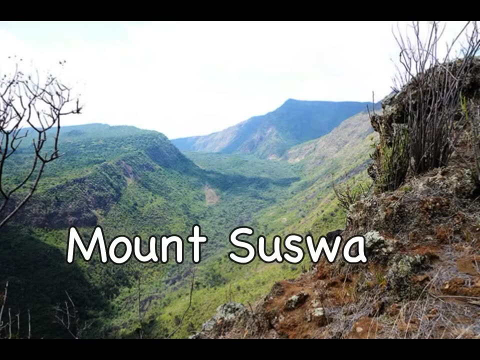 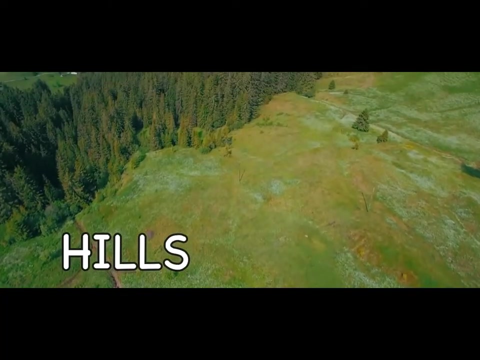 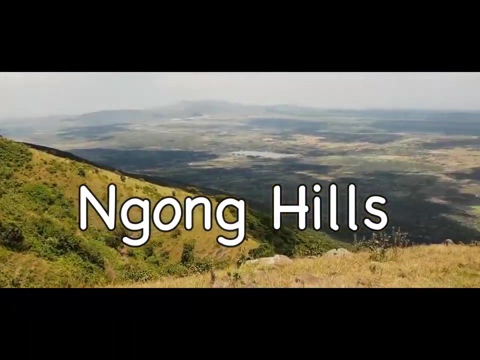 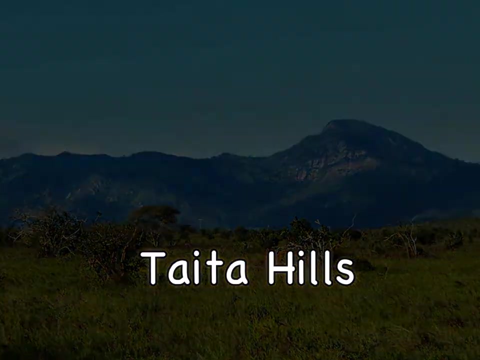 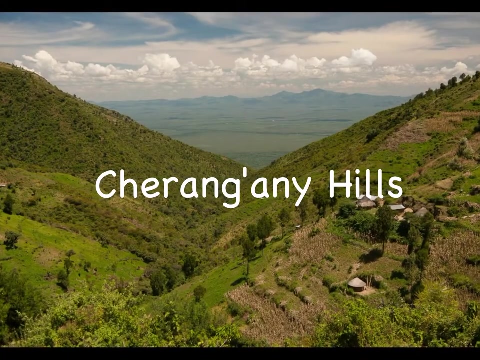 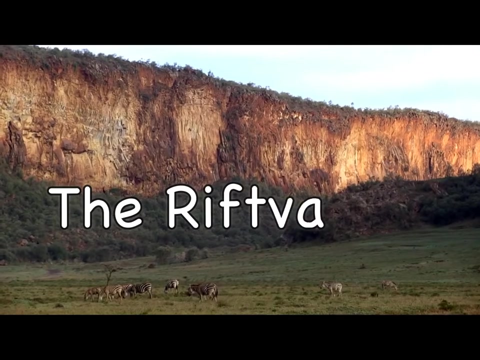 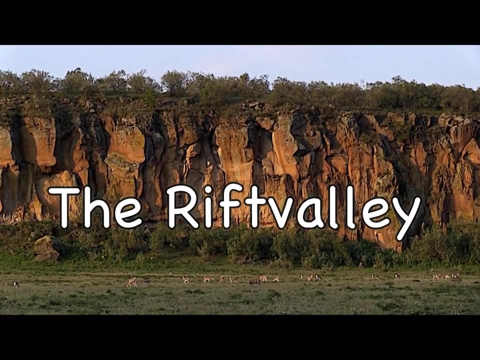 Mountordum, Mount Longornot, Mount Magritte, Mount Suswa, Mount Mersabit, among others Hills. Some of the hills include Ngong Hills, Taita Hills, Shimba Hills, Cherangani Hills and many others. The Rift Valley. The Rift Valley runs across the country from north to south. 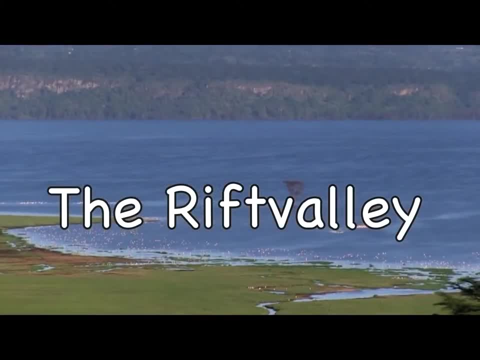 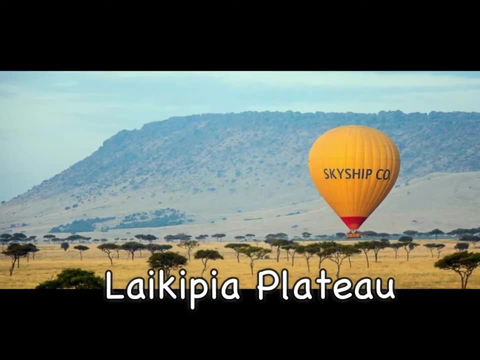 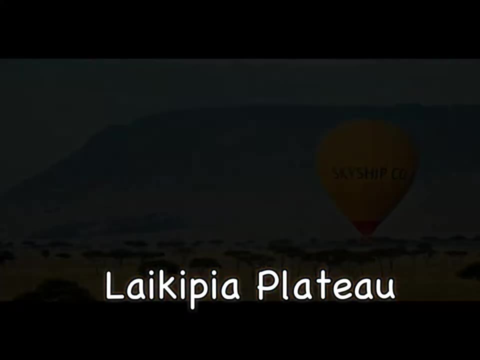 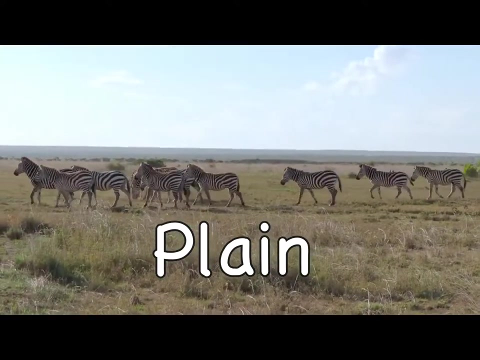 The Rift Valley is a hollow depression between highlands or mountain ranges. Plateau- A plateau- is a raised land that is usually flat on top. Example is Lake Kipia. Plateau Plane- A plane- is land that is flat and extensive. Example is Canoe Plane.